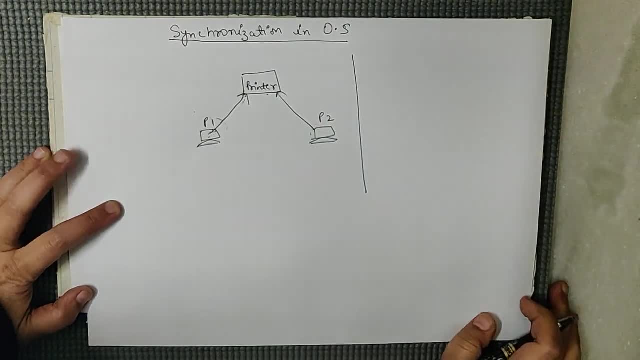 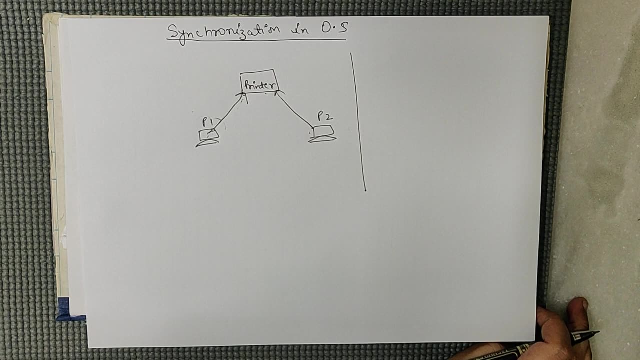 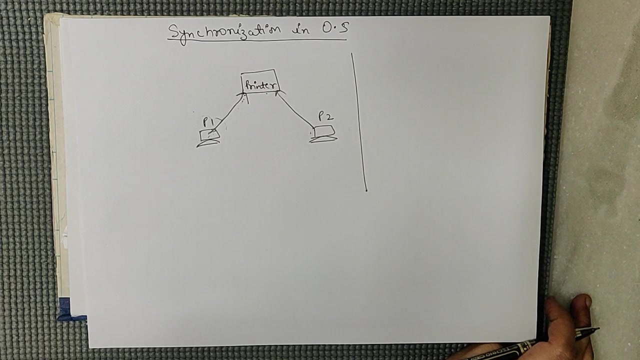 Okay, Also, I will give you another example. Say suppose, like you, people use the website of IRCTC railway. So when you мер 이거, What happens there is that the programmer on one side of the server is updating the time that which train will come and which train will not come. he is updating all the timings. 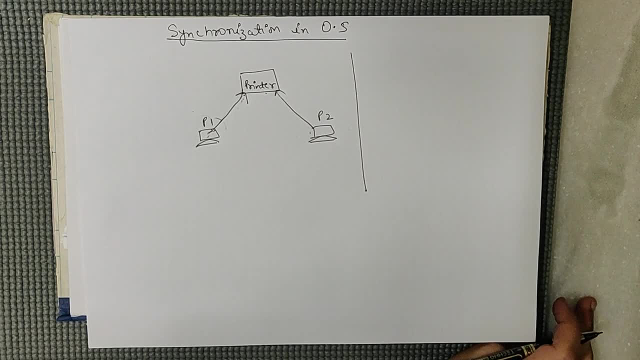 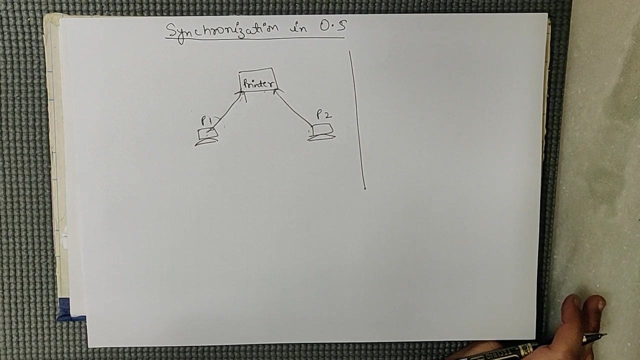 So until he doesn't update- now what is that website? IRCTC's website. what is that? It is a shared resource. So until he doesn't update all the timings of the train on the server, we as a user can't access the site, which means we can't see that thing which is not updated. otherwise, 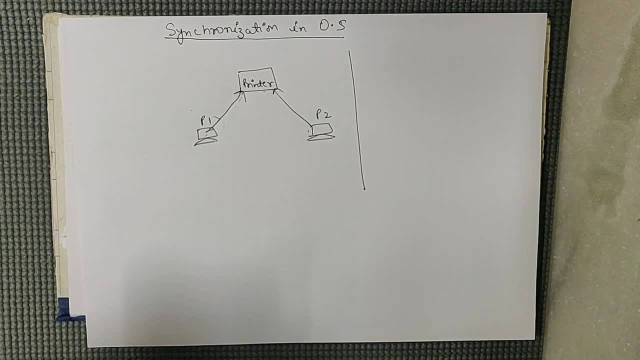 what will happen? We will get the wrong information because it is not updated from there and we are accessing it trying to read it. so it means it is blocked from there. now what message comes there? Update is still in process. the same message comes. if he does not display such a message. 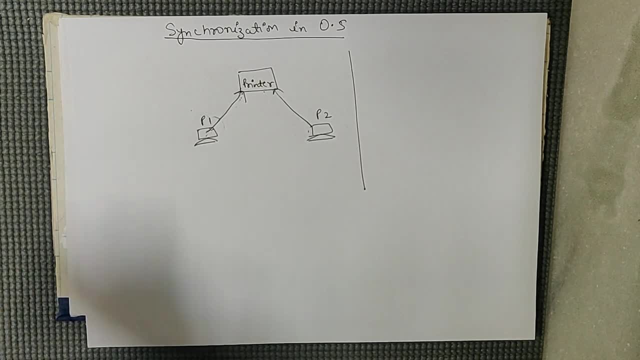 through programming. then what will happen? we will get wrong information again and again until the time, So the programmer on the server does not completely update him that which train is coming at what time, or how much time it is delayed, or how much time it is early. until then we 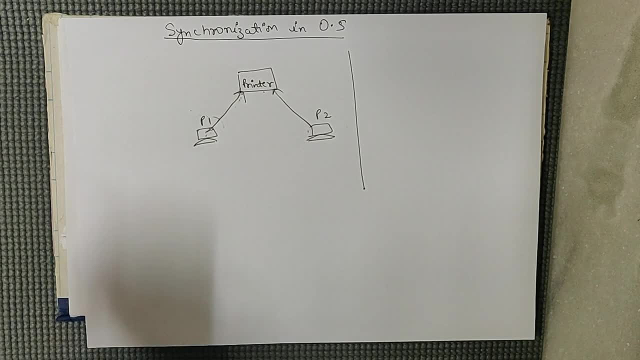 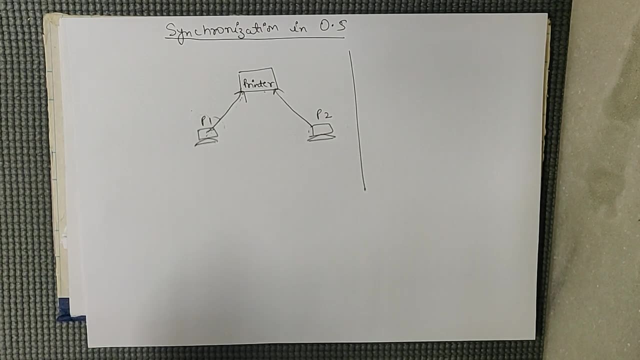 can't see the full timings of that site until then the update comes. update is still in process. He displays the message. holds it that at one time if the programmer is updating something on the server, then until he doesn't complete the update. we can't see it as soon as the 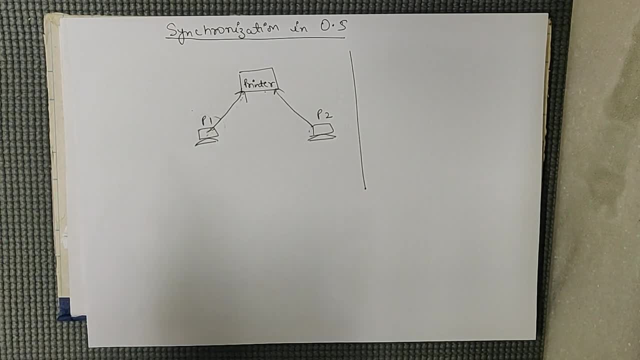 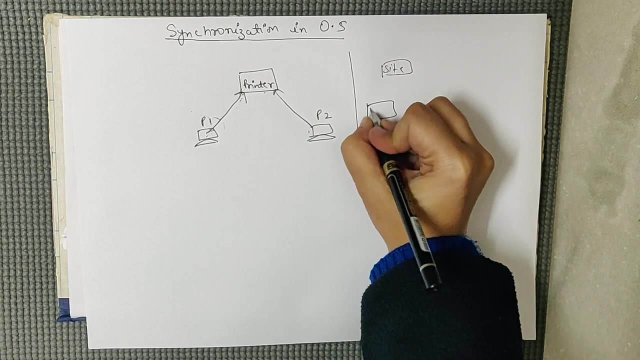 update is completed. after that, we get the chance to access the site. so what is the site? It is a shared resource. What is our site? What happened? Shared resource. Consider this programmer as a process. we are sitting here as a user. consider this. 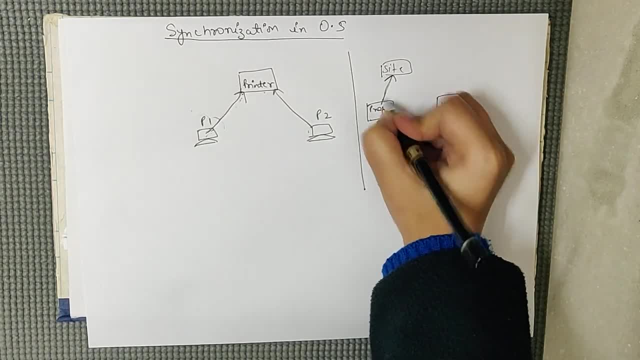 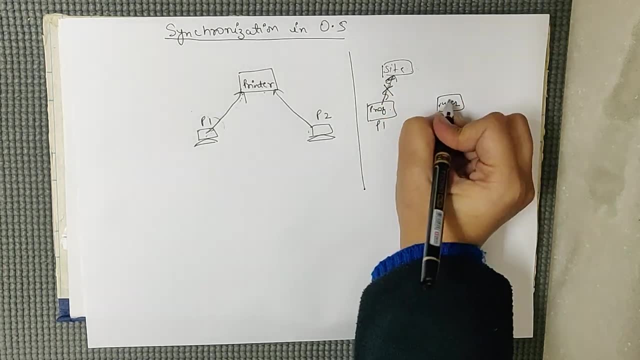 process as 2, so until he is accessing it, we can't access it. as soon as he has updated and he is not accessing it, there are no changes in it. then we get the chance to access the shared resource. So this is our shared resource.